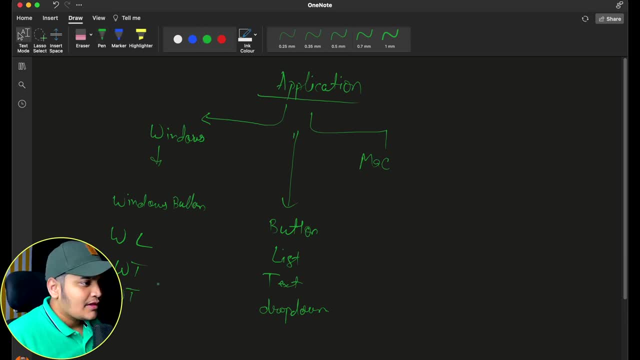 down, because that should be the proprietary for the Windows application- Windows one. but when I'm creating the application for my Mac, I want to use the Mac button, I want to use the Mac list, Mac text and Mac drop down list, which is proprietary to the. 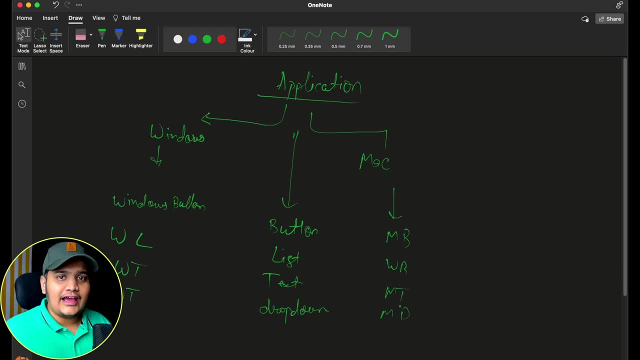 Mac application, As you already know that both these operating systems are different and based on that operating system, there'll be different UI components. Similarly, when I'm creating the application, I want to do the same thing Like whenever I'm going with. 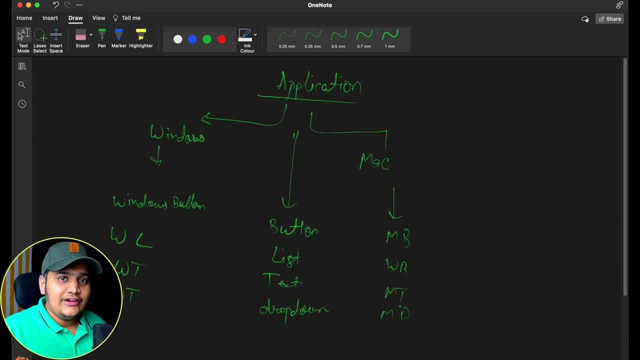 the windows. all those components should be loaded and should be added as per the windows application, as per the windows operating system. And whenever I'm going with the Mac, all the components should be with the Mac operating system. Okay, So here I can say: 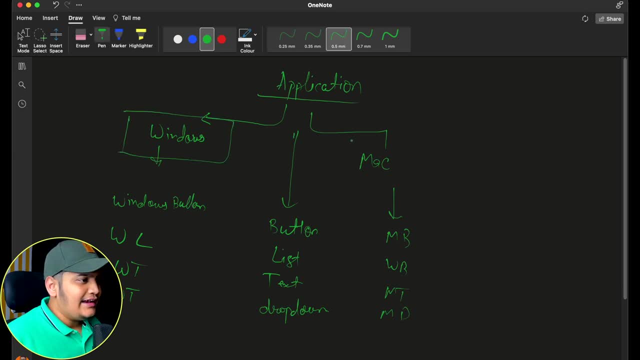 this is one of the factories that it will create the windows application for me, And there is one more factory, that is the Mac UI application factory, which will create the Mac UI application for me, And this application is the another factory. that is the abstract. 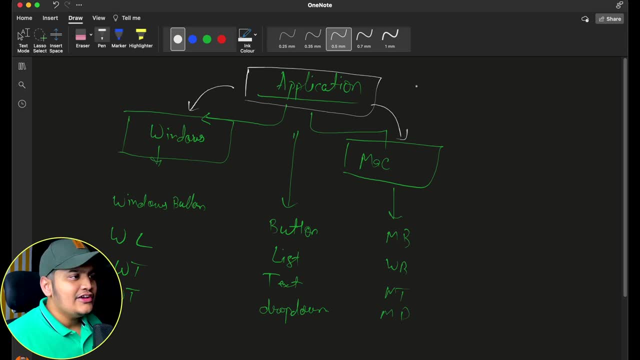 factory on top of the Mac factory and the windows factory, which will create the applications. Okay, So whenever I want to create the application, I can just tell that, okay, I want to create the application, which application? I want to create the Mac application? Okay, So I'll. 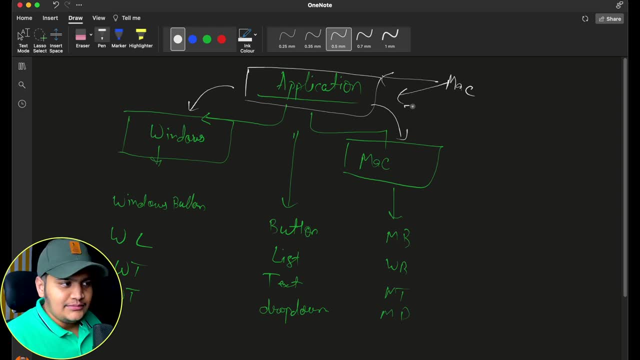 just pass that I want to create Mac application. It will again, in terms, go to this Mac application. it will create the classes for it And it will also create these similar classes for this UI components as well. Okay, So this Mac will not go to create the components based. 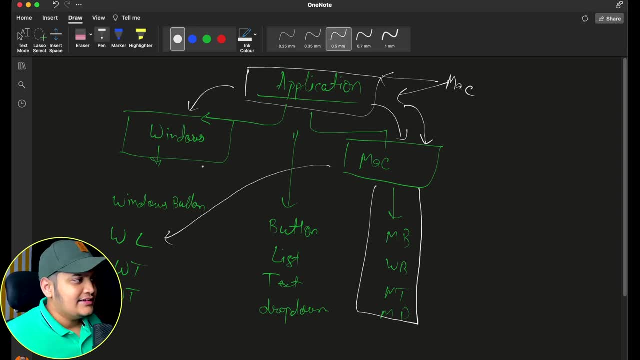 on the windows. It will only create based on the Mac. Similarly, when I'm going with the windows, it will go to create the windows by default and setting it to one like thisiest version. So it will not come up with the terms of the tools at having that features Moving. 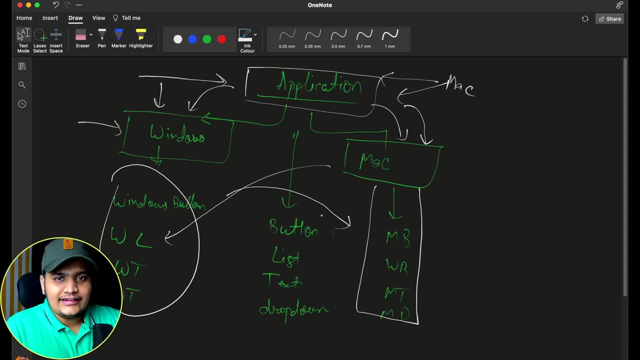 ahead and telling these application that I want to create the windows application. it will, in terms, again create the windows application and it will lower this components, only It won't load this components. Okay, So you can see that I have the abstract factor, that is. 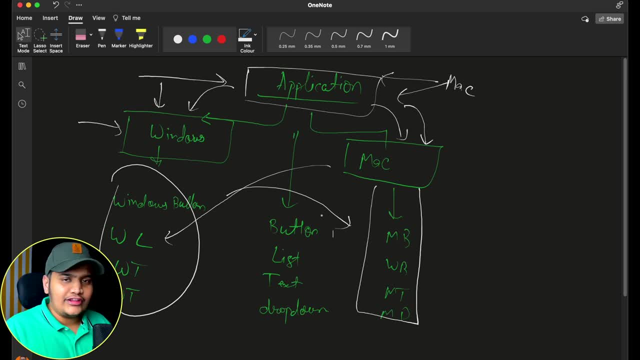 the application and within that application I can define: okay, I want Mac or windows and, accordingly, all those Okay factories that we have designed. so let's see this by example, how we can implement this. so let me go to my intellij idea. okay, and here you can see that i have created some of the classes. 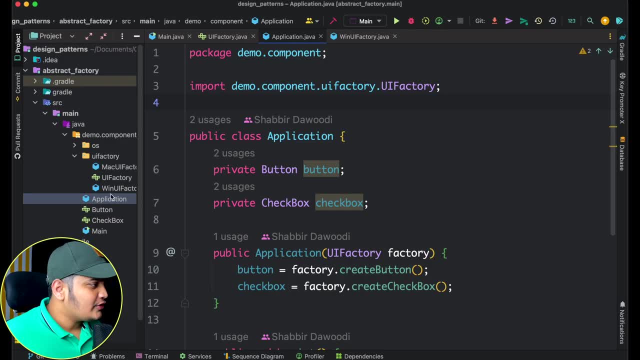 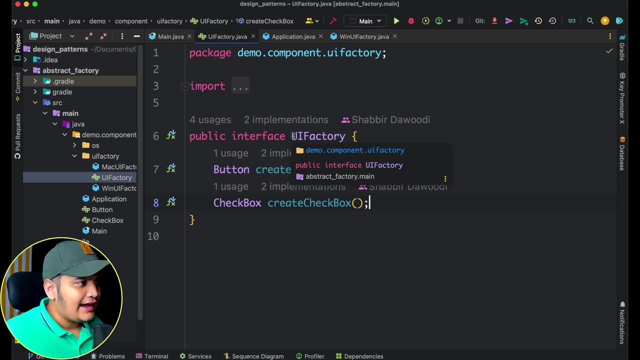 which will depict the same thing that we have explained here. so here you can see that i have few of the classes, okay. here you can see that i have ui factory- okay, and this ui factory is the interface. and this ui factory may contain two methods, that is, the create button and create. 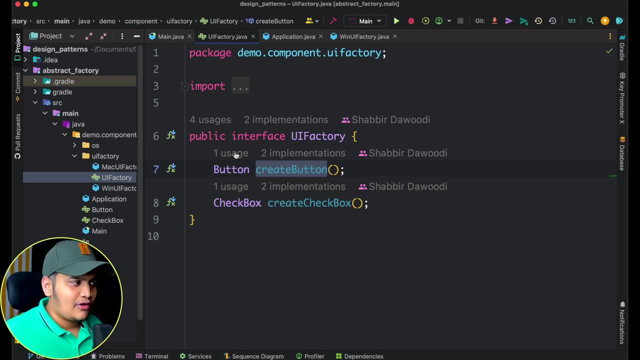 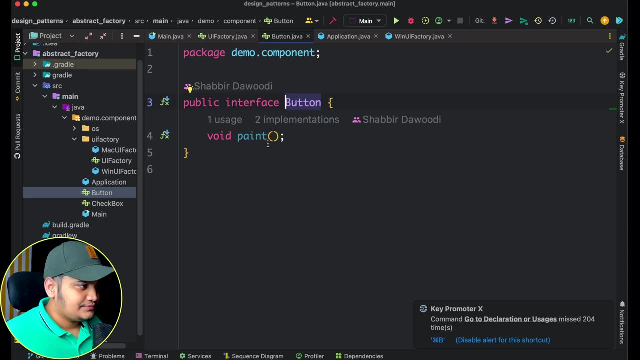 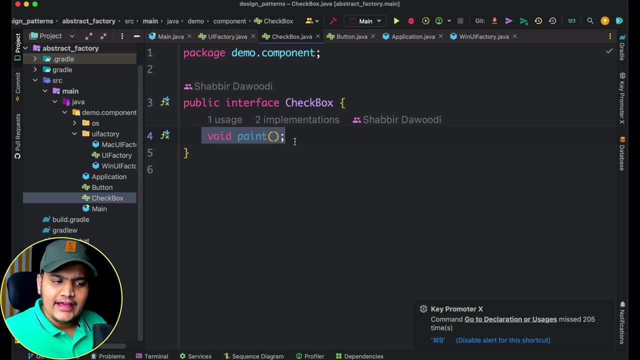 checkbox button. okay, two methods to add the button and checkbox. and this button and checkbox are again the interfaces. okay, this is a standard button and a button is painted and we have a checkbox and that checkbox is also interface and which is going to be painted in the application. 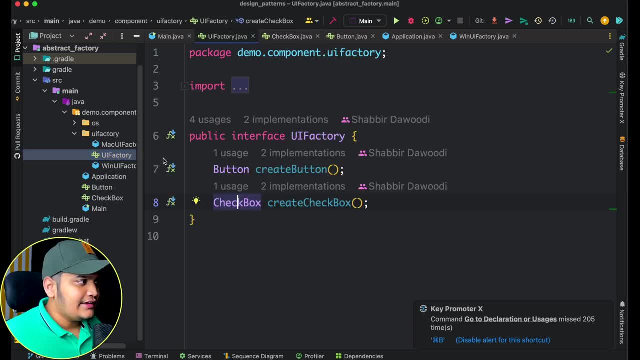 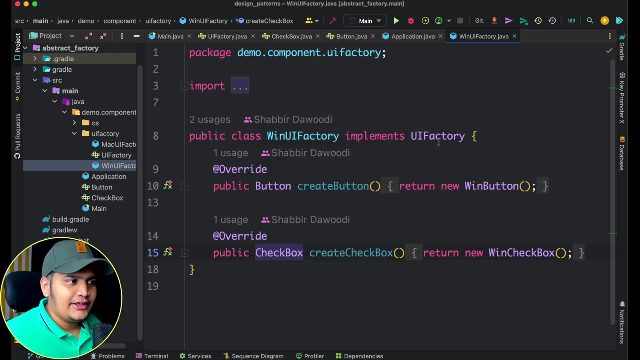 okay, two simple things now. my this ui factory is implemented by the windows ui factory. okay, you can see that this windows ui factory is a class that is implementing ui factory and we have implemented two methods, that is, the create button and the create checkbox button, and you can see this will return the windows button we have created. you can see if you go. 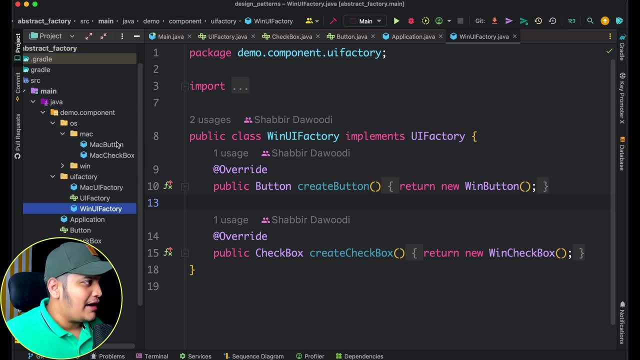 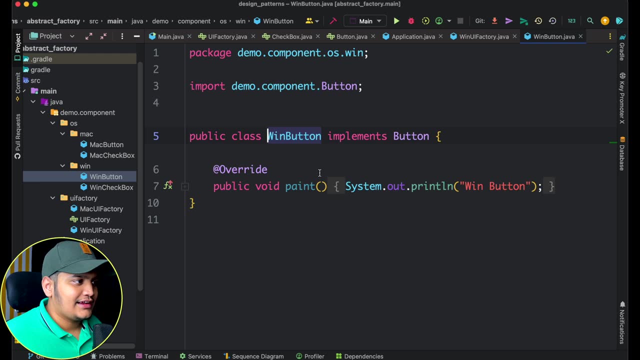 to the os and within the mac i have mac button and mac checkbox and within the windows i have windows button and the windows checkbox. you can see these two proprietary buttons are there right? you can see windows button is again implementing the button that is going to say: this is a windows. 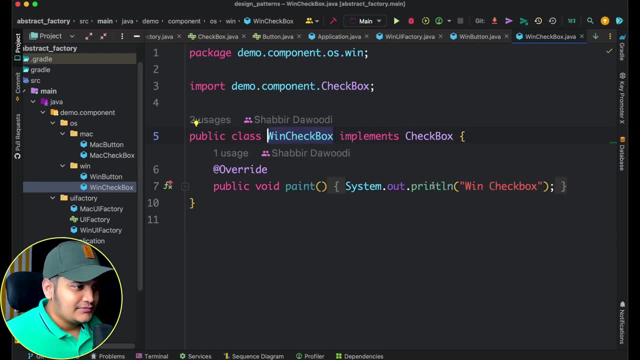 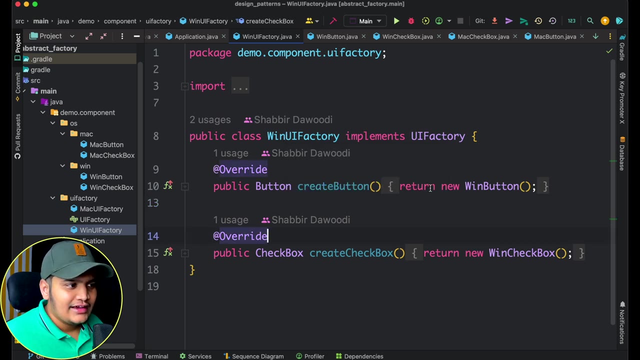 button and windows checkbox is going to say: this is the windows checkbox, similarly Mac checkbox and the Mac button. So this you can see. the components are different and this component will be loaded based on the UI factory. So within the Windows UI factory you can see we are passing return, new windows button and 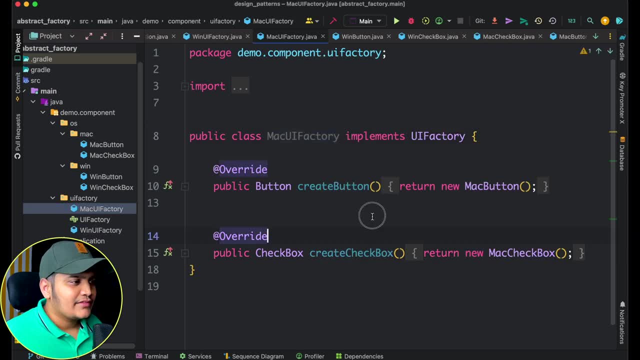 return new windows checkbox and within the Mac UI factory we are passing within the same implemented method, that is, the create button and the create checkbox, and within that we are passing return Mac button and return checkbox button. So ideally, whenever I have the object of Mac UI factory, that will give me Mac button and 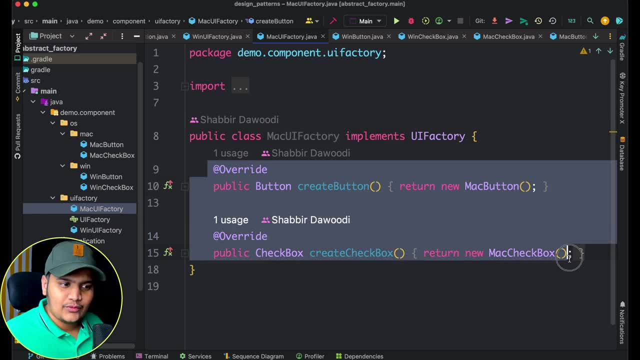 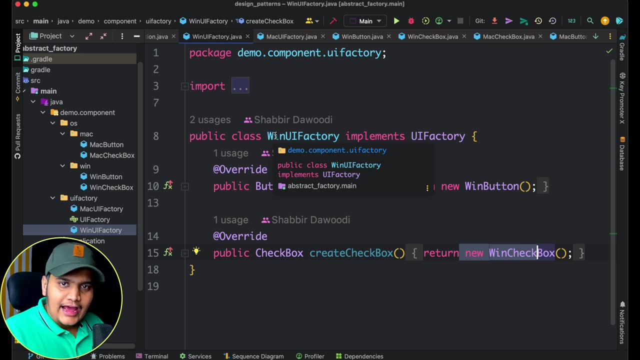 Mac checkbox by default. right, because we have the implementation that way. Similarly, when I have the object of WinUI factory, I will get the button of Windows and Windows checkbox only because we have implemented that way. So that factory layer is then that based on the individual factory, either it's Windows. 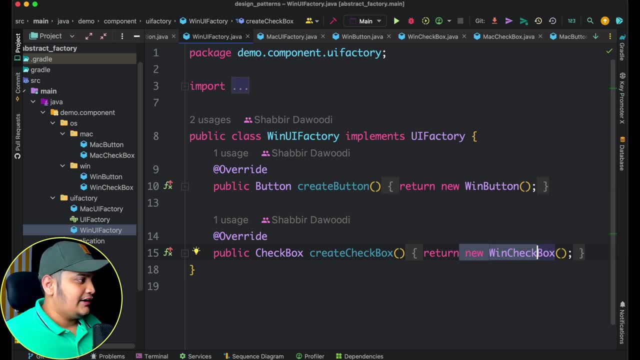 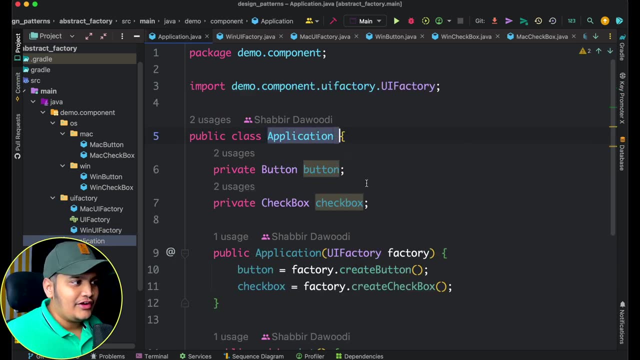 and Mac. I will get the supported UI components Now if I go to the main application, that is, the main factory itself. Okay, so this application and within this application, we have defined that this application will contain button and checkbox, because all our applications should contain button and. 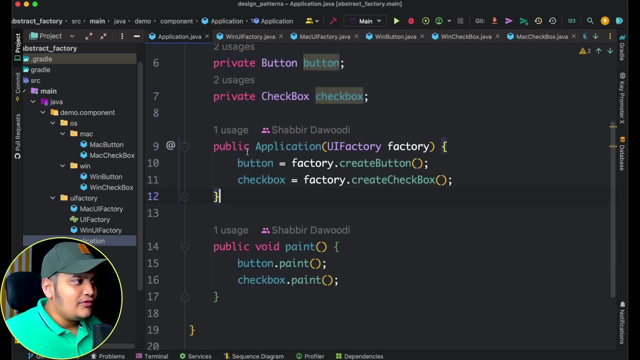 checkbox. okay, and we have created a constructor here. okay, and this constructor is taking the UI factory. okay, that is the another factory. okay, that's the UI factory. Now, within this factory, you can see that we are calling factory dot- create button and factory dot- create checkbox. okay, and we are calling those methods. 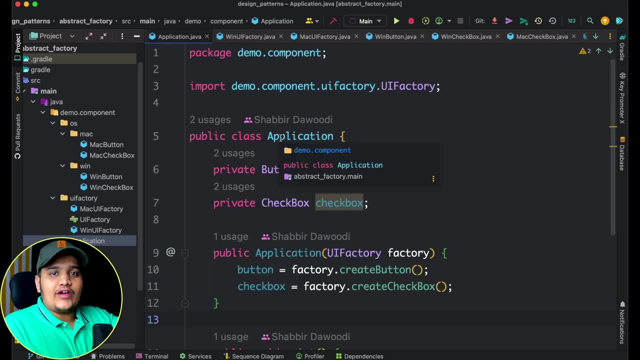 Simple thing. okay, So you can see that this application, that's the factory of factory, that is just taking one input. give me the factory and what I want to do, okay, So here you can see, we are just taking the factory and from that factory, whatever the 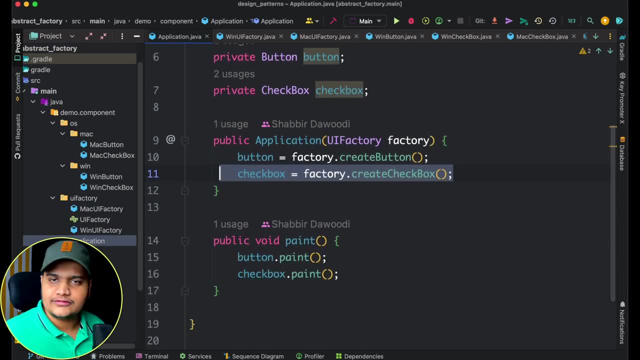 methods are available, those methods we are calling and setting those values, simple thing. okay, Now how we will call this? actually, okay, so if you go to the main method, okay, and here you can see that we want the application to be created. okay, in the main method we have. 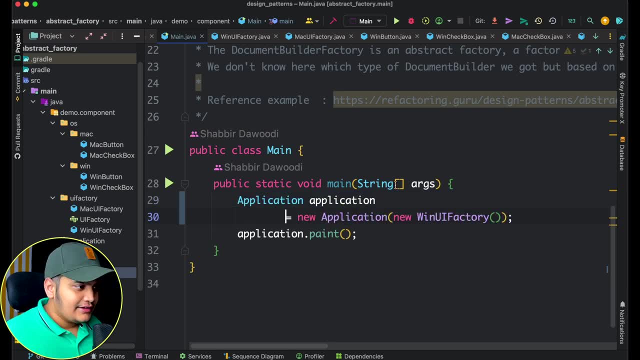 defined that We want the application to be created and it's going to be the new application. and within this new application we have the constructor, where we have passed the UI factory and we want to pass the implementation of the UI factory. so we pass that win UI factory, okay. 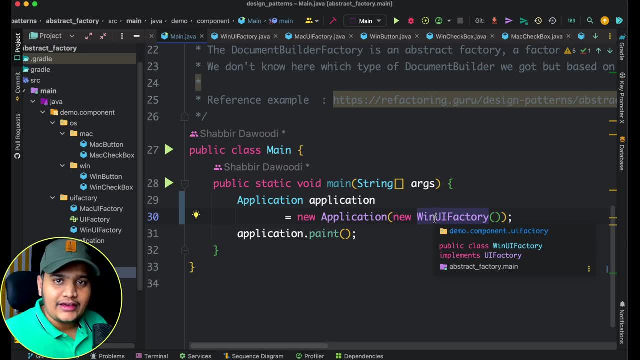 So now all the components of the Windows UI will be created and that will be displayed here. okay, So you can see we created an application that is the factory of factory. within that we pass that. we want UI factory. okay, Which UI factory? Windows UI factory? 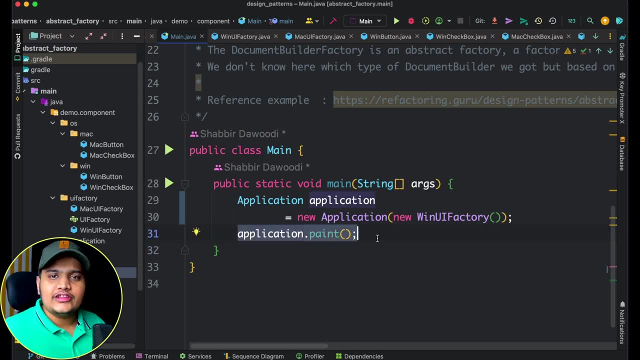 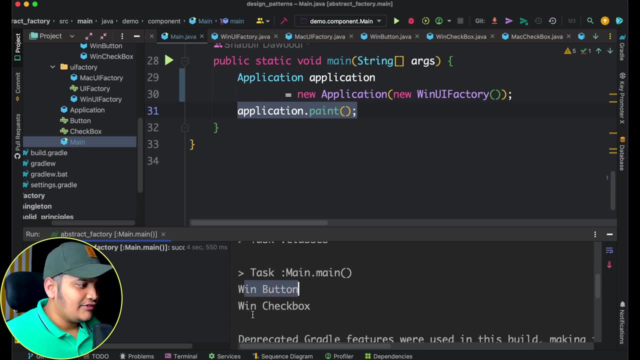 So now, whatever the applicationpaint we will do, everything will be based on the Windows. so if I run this, you can see that we got the Windows button and we got the Windows checkbox. okay, We have not added any conditional checks or anything anywhere. okay, based on the object.